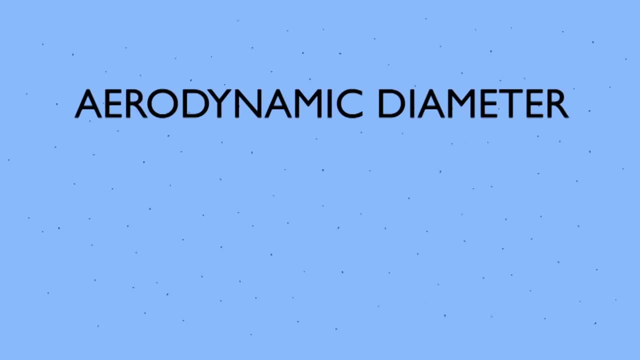 These particles are identified, according to their aerodynamic diameter, as either PM10- particles with an aerodynamic diameter smaller than 10 microns- or PM2.5. These have aerodynamic diameters smaller than 10 microns. In comparison, the average size of a human hair is 60 microns. PM2.5s are more dangerous. 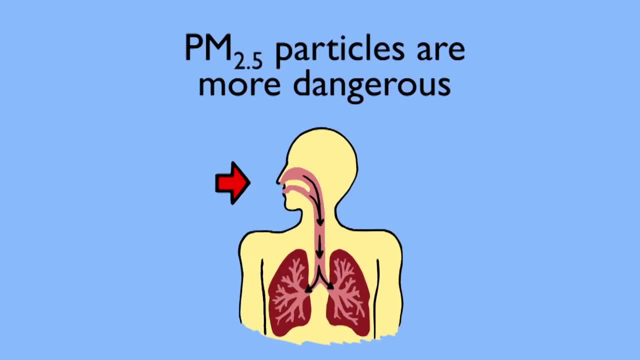 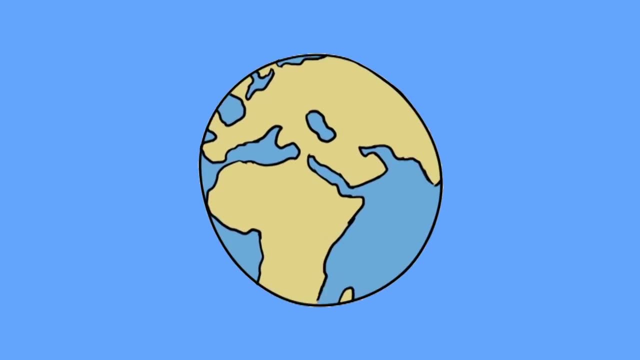 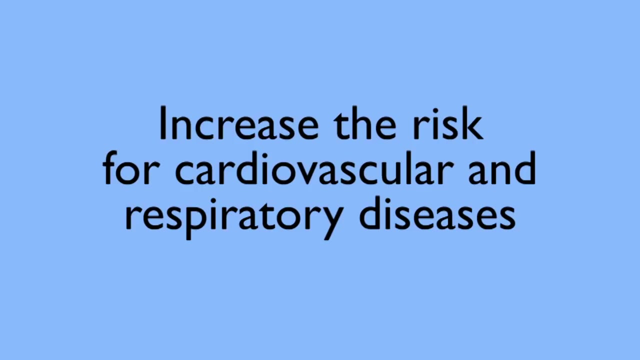 since, when inhaled, they may reach deep into the lungs and interfere with gas exchange. The health effects of particulate matter are felt in both the developed and developing world. Chronic exposure to particles contributes to the risk of developing cardiovascular and respiratory diseases. 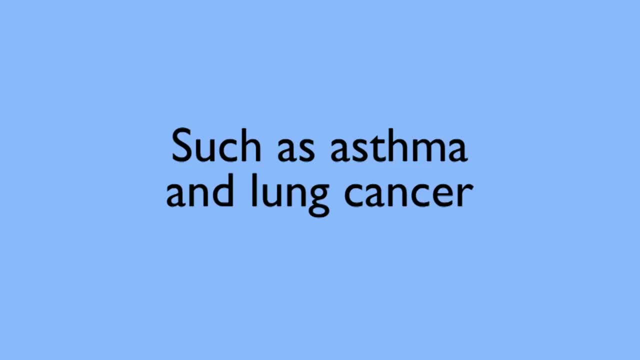 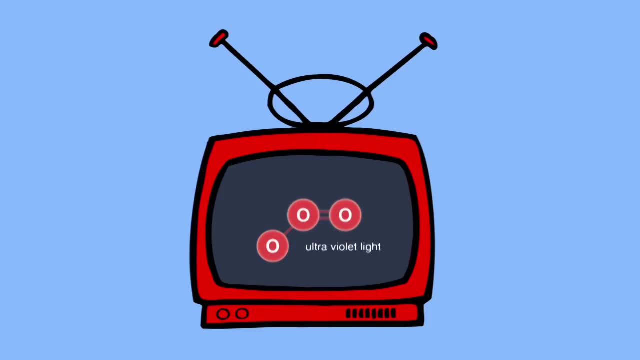 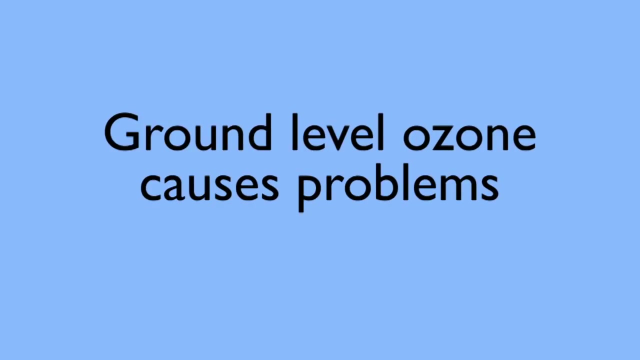 Ozone O3, absorbs harmful UV rays from the sun in the upper atmosphere and can help prevent the increased risk of skin cancer. However, ground-level ozone causes problems. It does so by a photochemical reaction which is triggered by the absorption of light. The reactions 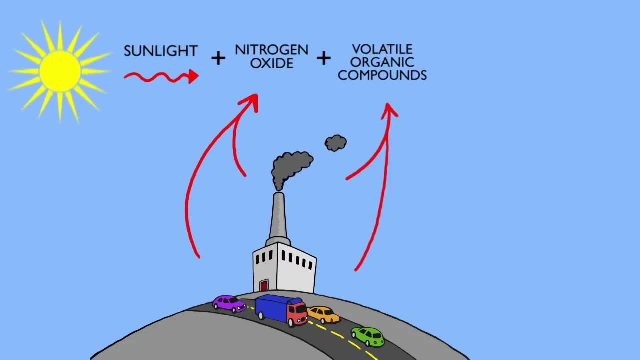 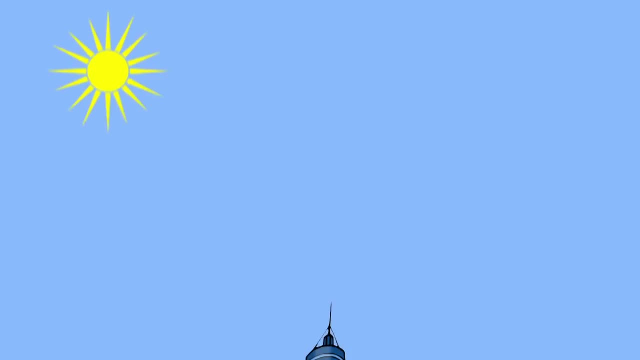 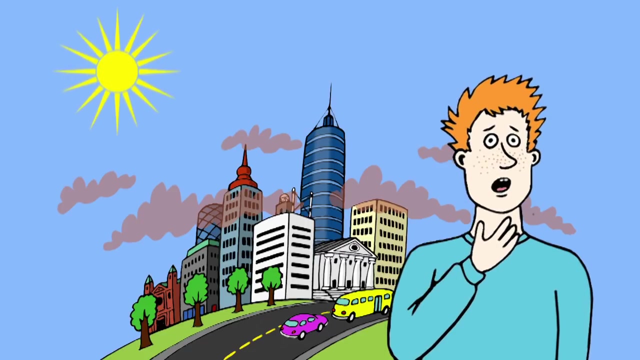 between nitrogen oxides and volatile organic compounds lead to the formation of a photochemical smog and ground ozone. You see this more often in the summer and it can appear as an orange-brown haze over a city. This smog, including the ground ozone, causes breathing. 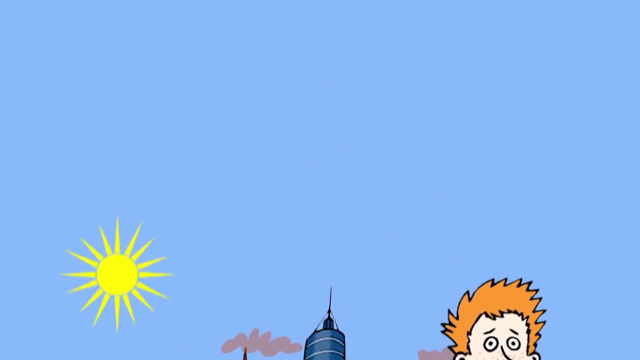 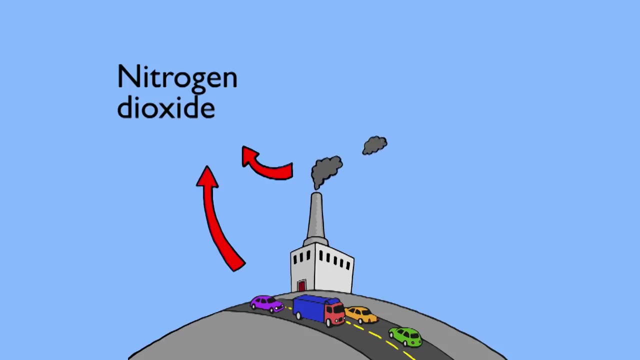 problems can trigger asthma attacks and lead to lung disease. Next, nitrogen dioxide emissions come from cars and factories where fuels are combusted. You may recall, oxygen forms about 21% of our atmosphere, whilst nitrogen forms 79% of our atmosphere. This is due to the fact that oxygen forms about 21% of our atmosphere. 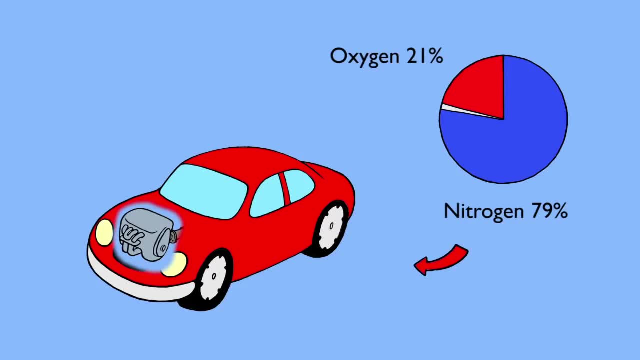 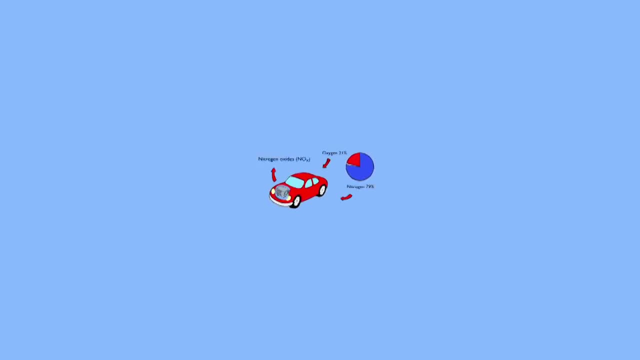 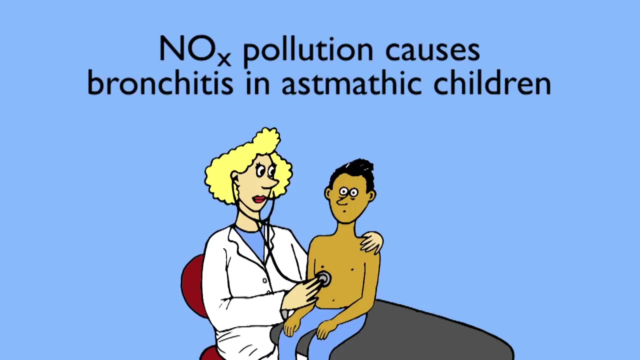 whilst nitrogen forms about 20% In a hot engine, a tiny amount of nitrogen atoms join with oxygen atoms to form mixtures of nitrogen oxides called NOx. Studies have proven that there is a causal relationship between the symptoms of bronchitis, a respiratory disease. 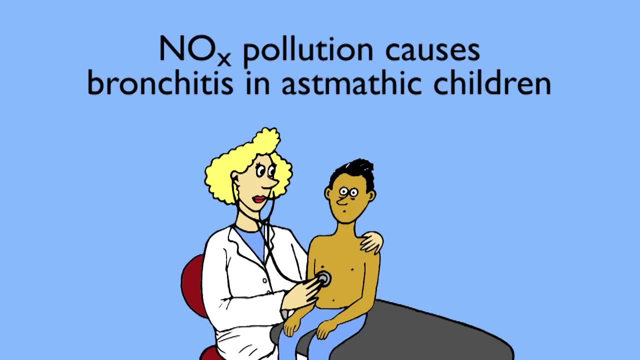 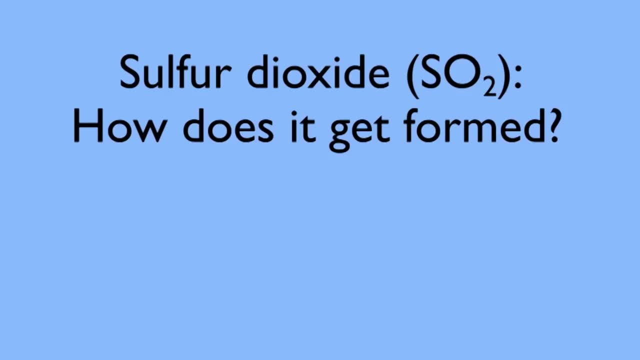 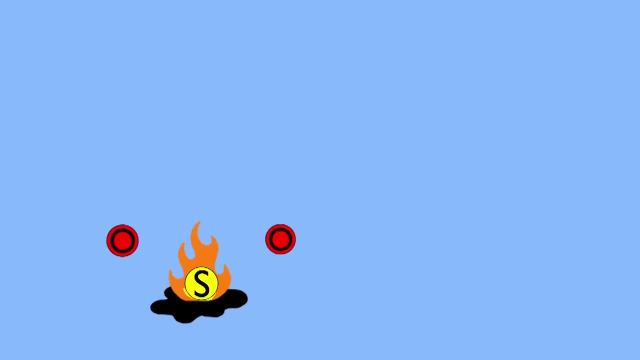 being seen in children with asthma as a result of long-term exposure to this pollutant. Finally, there is sulphur dioxide. Can you think how this chemical might be formed? Pause the video and continue on. The correct answer is that any sulphur combusted in the presence of oxygen, typically coming.